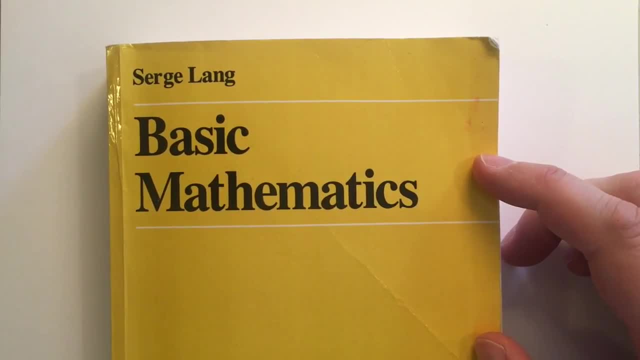 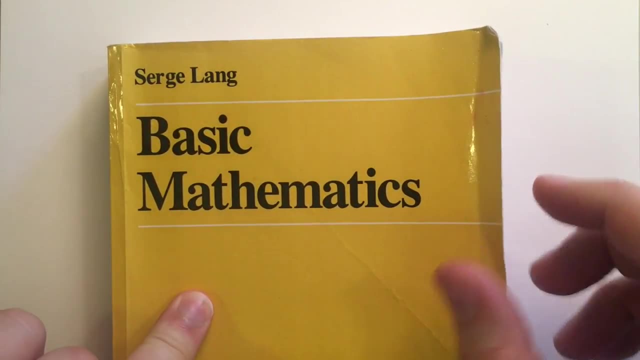 Hey guys, this is Jonathan Gardner. Thank you for watching me on Real Physics here. This video series is going to be on Sergey Lang's Basic Mathematics. You can pick this up at amazoncom. I'll provide a link. Obviously, it's a paid link, a sponsored link, And this is a great 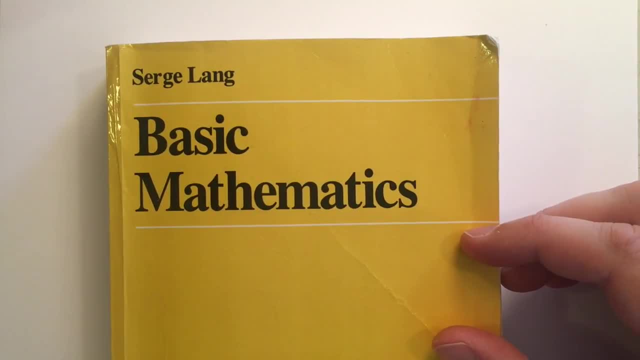 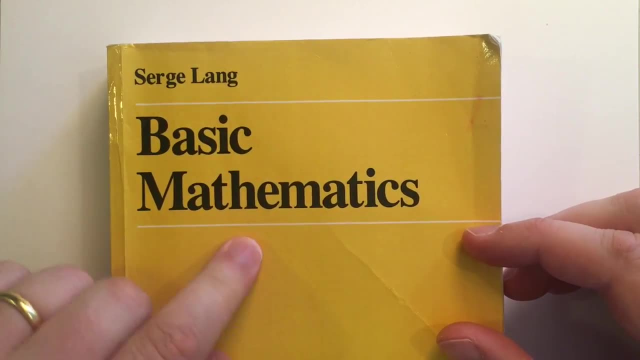 book for getting back into mathematics. if you've been exposed to arithmetic, you know some basic geometry, basic algebra, and you want to get up that level while you're ready for calculus. This book was introduced, I believe, back in the 70s to address the problem that many high schools 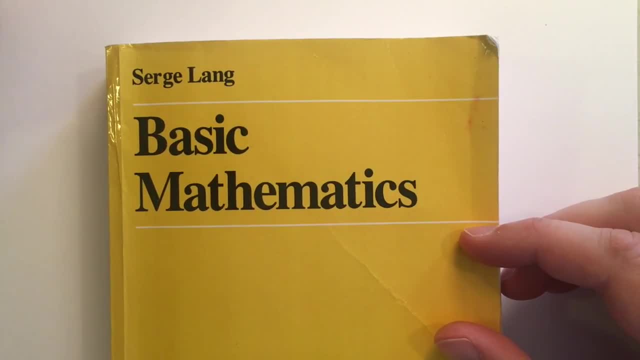 weren't teaching calculus and advanced mathematics, or they were teaching in an inconsistent way, And so this book was designed sort of as a remedial text to get college students ready to learn advanced mathematics and become future mathematicians. You'll note that this book 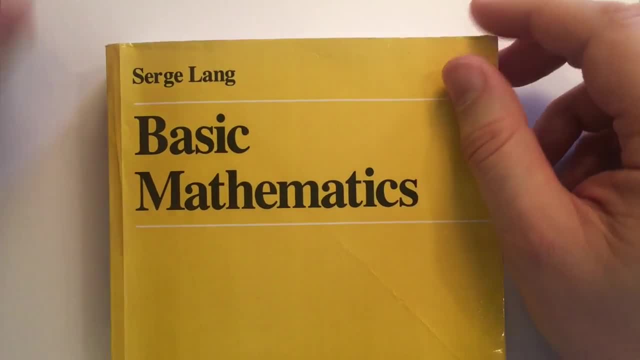 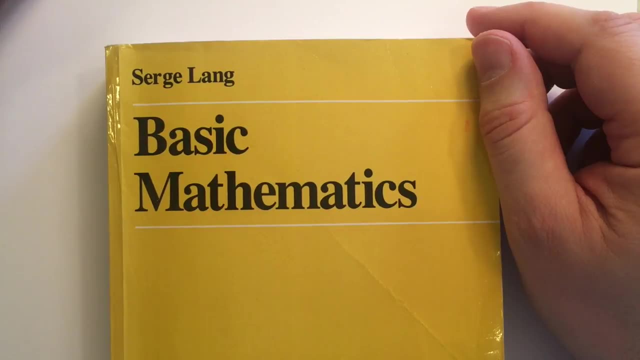 is. it doesn't have a lot of pictures. It's very dry. The focus of this book is to get you into the math, experimenting with the formulas and theorems, and to try to start learning how to make your own theorems using logical reasoning and things like that. So this is definitely a 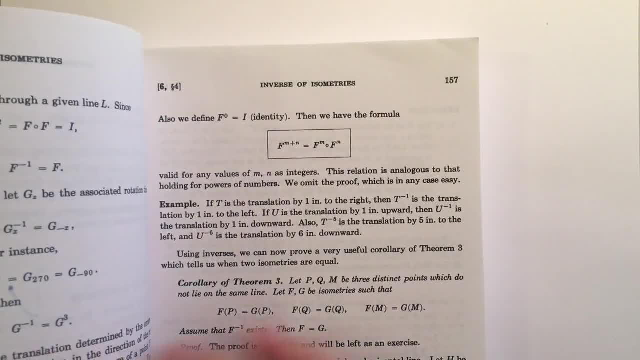 book that I'm going to be using a lot of my time. I'm going to be using a lot of my time to where you have to go in there and try to solve the problems on your own and give yourself, give your brain, a chance to learn more about how math actually works. Eventually, you're going to 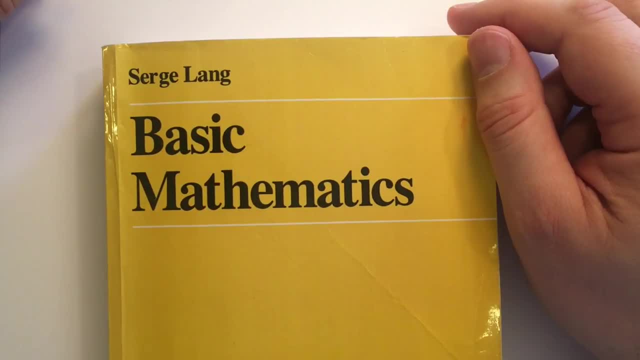 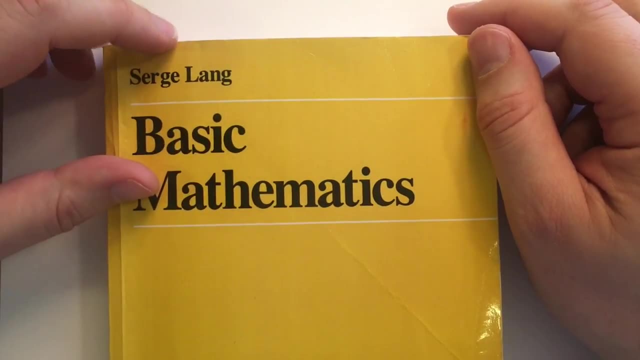 reach a point in mathematics where there just aren't any new problems to solve. From here on out, we're going to teach you how to solve problems, how to solve the problem of problem solving. I don't know if I said that right. Basically, you're going to learn some techniques to solve any kind. 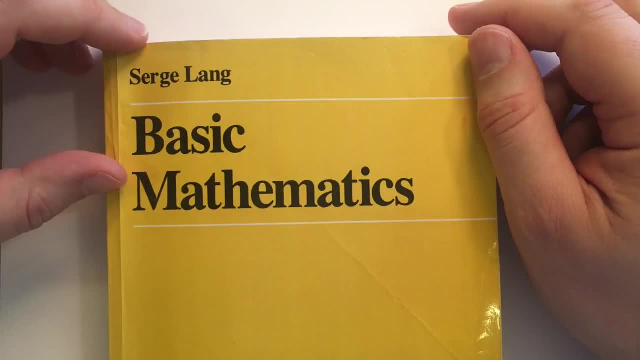 of mathematics problems, And once you start mastering those techniques, you'll realize there just aren't many problems to solve. And so this book is going to be a book that you can use, because some people will say: what else is there to solve than just solving other problems? that 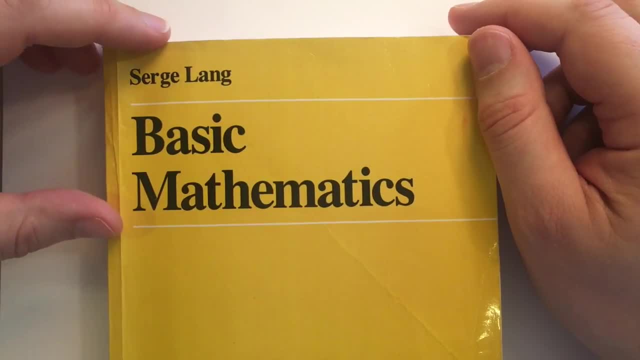 you can't solve yourself, And so that's where I'm coming in today. in this book, I'm going to show you my old background. This is where you can start to find some things to besz, And it's a lot like math or algebra, where you'll get a lot of algorithms. You'll have to keep gathering. 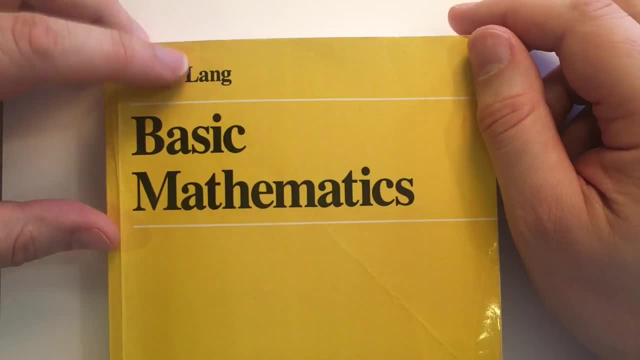 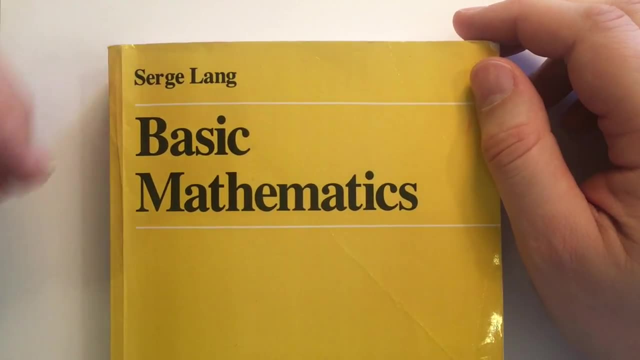 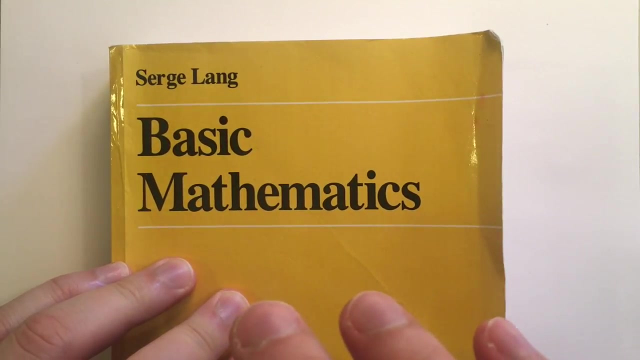 ideas and learn other things. Basically, I'm going to include several concepts for you to explore and use together for your own CANS and interesting yoga tasks, andЖ¯ Haused Practices, La Liga, which was one of the collectibles that I designed. So what I'm going to do now is I'm going to place some of the